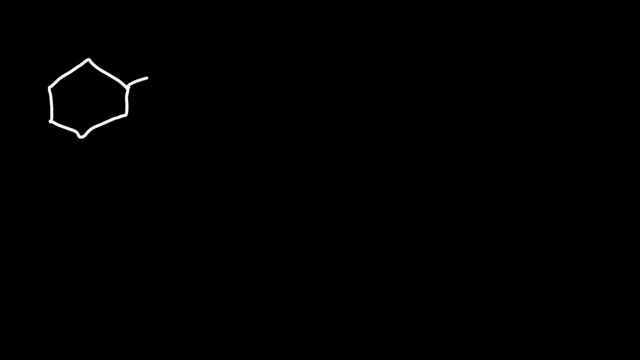 Now let's move on to our next example. What is the name of this molecule? What's the parent name? Now, we can also write it like this too. So instead of CHO, it's going to be C, with a double bond O and a hydrogen attached to it. So we have a benzene ring. We're going. 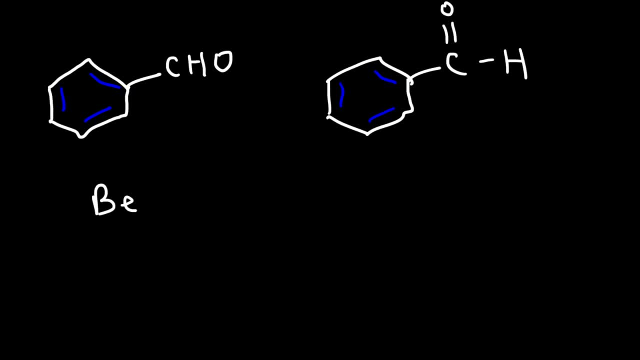 and an aldehyde functional group. So this is going to be called instead of benzene, it's benzaldehyde. Now what is the common name for this molecule? Let's say, if we have a benzene ring and a carbon-carbon double bond attached to it? 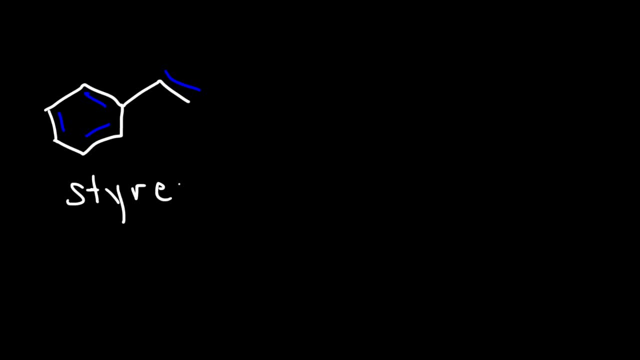 The common name is styrene. This is also called veno-benzene, because this is a veno group. Now what if we have a ketone next to a benzene ring like this one? This is called acetylphenone. 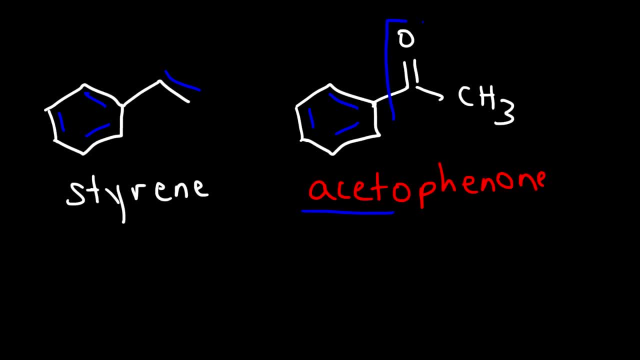 When you hear the word acetyl, think of two carbons. This is the acetyl, This is the acetyl group. And then when you hear the word phenol, phenol has to do with a benzene ring with six carbons. 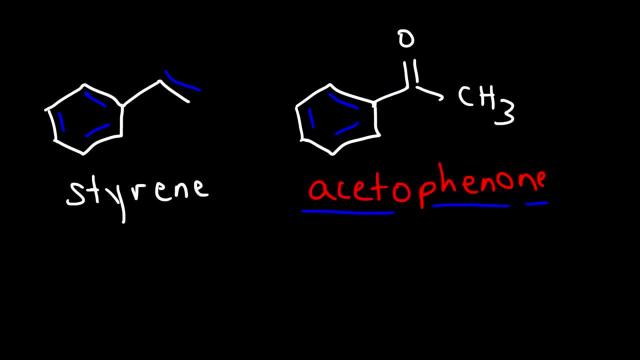 And the one tells you we're dealing with a ketone. Now what if we have a halogen attached to a benzene ring? So let's say, if we have a chlorine atom compared to a bromine atom, How can we name these two benzene derivatives? 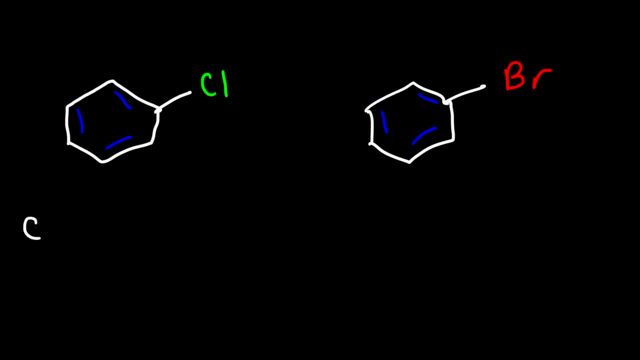 So for the molecule on the left, this is called chlorobenzene, And for the one on the right, you can guess what it is That's going to be called bromobenzene. Now what if we have an ethyl group attached to a benzene ring? 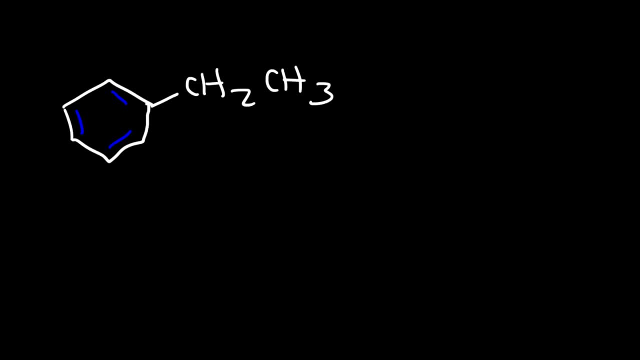 What's the name for this molecule? Now, this one is pretty straightforward. This is simply called ethylbenzene. That's it for this example. Now what if we have a methyl group attached to, let's say, a benzene ring? 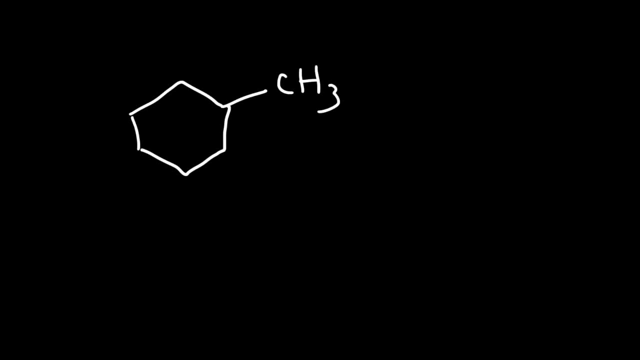 So what's the name of this one? Can we say that it's methylbenzene? That would make sense. But this one has a common name that you need to know And it's called toluene. You'll see that one. 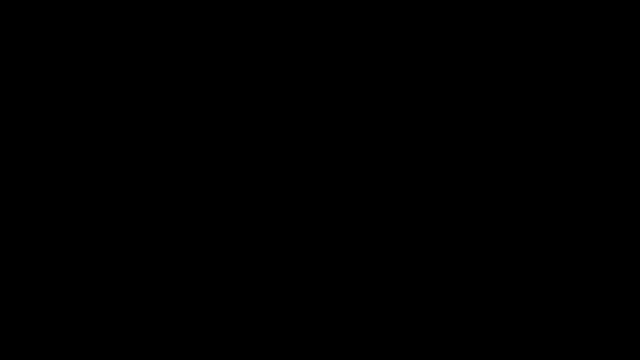 So make sure you know this common name. Next up, we have a benzene ring with an amide functional group. So what's the name for this molecule? So benzene plus an amide. this is called benzamide. Now what if we have a benzene ring? 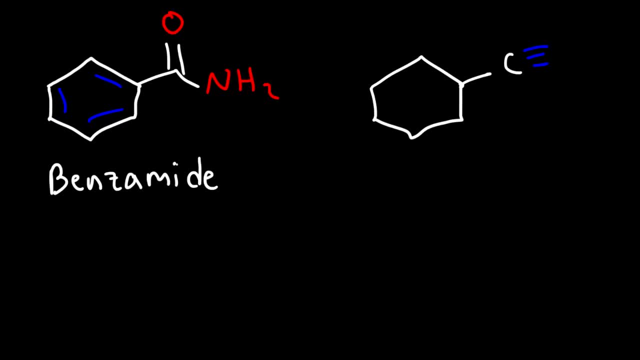 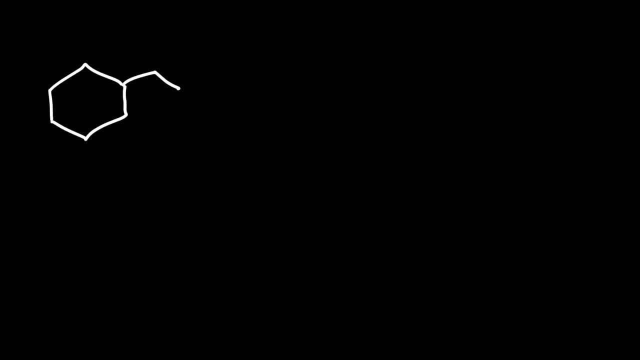 Now what about having a benzene ring and a ch2 group, followed by a chlorinated one, chlorine atom? What's the name for this molecule? So this is a phenyl group if it's just the benzene ring, But the phenyl group plus this extra carbon, which? 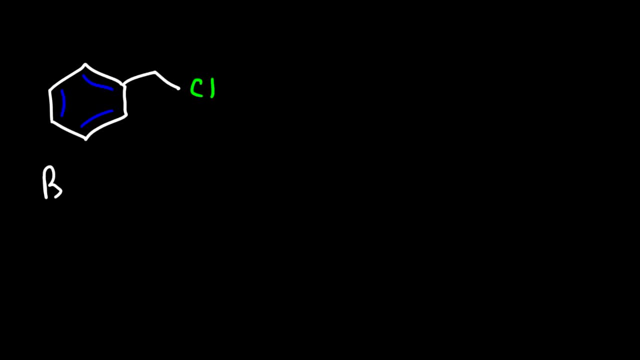 totals seven carbons. that's called benzyl, And so this is called benzyl chloride. So remember, a phenyl group has six carbons. a benzyl group has seven carbons. It has the benzene ring plus this additional carbon. 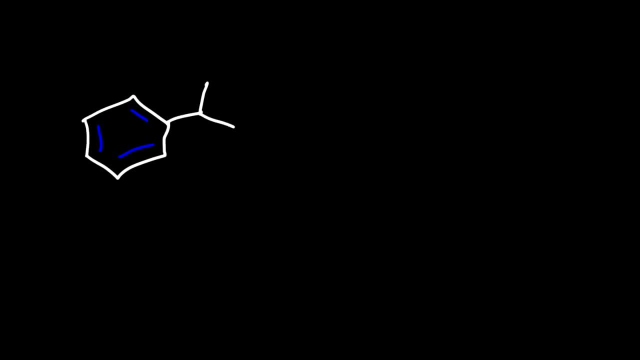 Now what about this one? How can we name this molecule? So here we have an isopropyl group, And so we can call this isopropyl benzene. It also has another name. The common name is cumene. So if you see cumene, it's not cumene, but cumene it's isopropyl benzene. 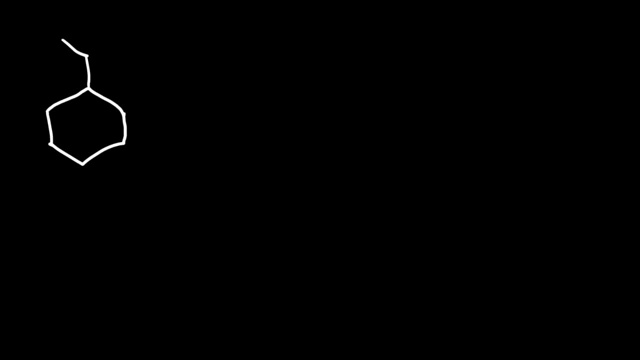 Now let's move on to our next example. So here we have a tert-butyl group attached to a benzene ring, And so this is going to be called tert-butyl-benzene. Now what if we have a benzene ring attached to a sulfur atom that has two? 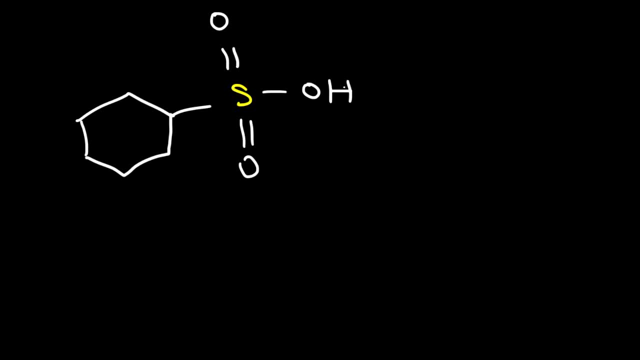 double bonded oxygen atoms attached to it and an OH group. So if you see this group, this is called a sulfonic acid. Combined, this is benzene sulfonic acid, Kind of like a carbo, like a carboxylic acid, but instead of that it's a sulfonic. 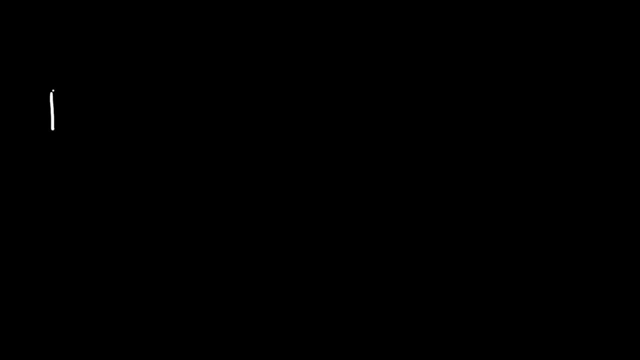 acid. Now let's move on to name in disubstituted benzene derivatives. So we saw that if we have one methyl group, it's called toluene. What if we have two methyl groups attached to a benzene ring? How is the name going to be different If? 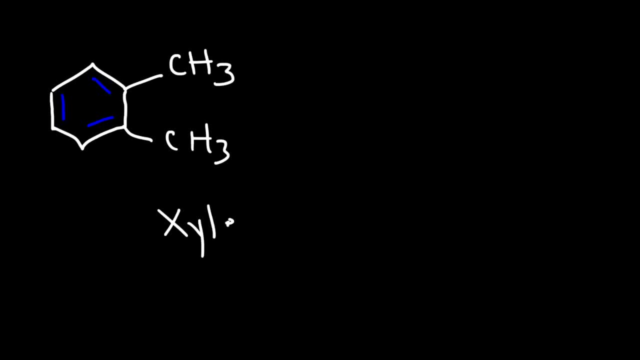 you have two benzene- I mean two methyl groups rather- attached to a benzene ring. you're going to have two methyl groups attached to a benzene ring. It's going to be called a xylene. Now this specifically is known as ortho xylene. 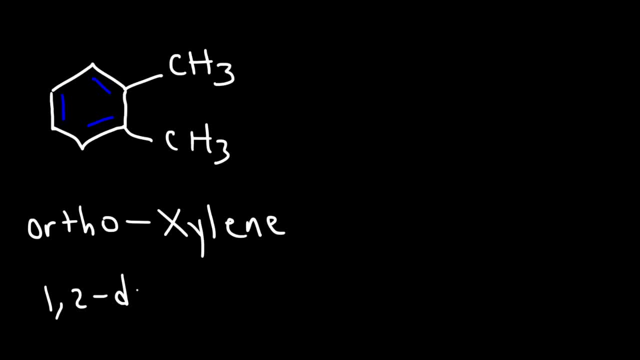 It's also called 1,2-dimethylbenzene, So let's call this carbon 1.. This will be number two, three and four. So with respect to the first methyl group, the second methyl group is at the ortho position. 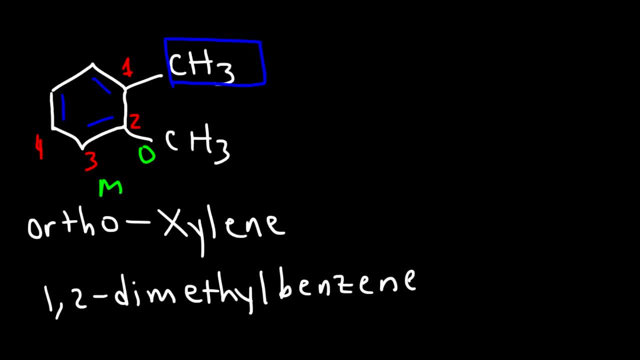 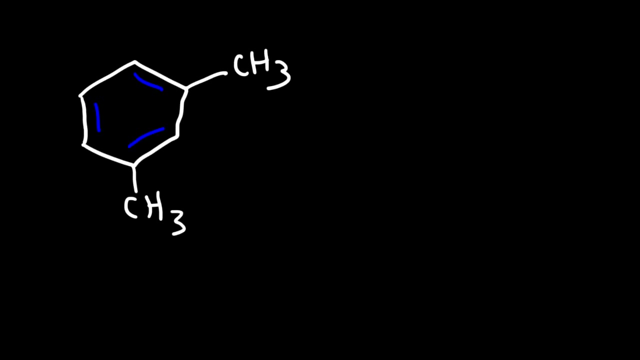 Ortho is 1,2.. Meta is 1,3.. Pera is 1,4.. Now, what about this example? What is the name of this molecule? Go ahead and try. So this is still going to be xylene, but instead of 1,2, it's 1,3.. So we can call. 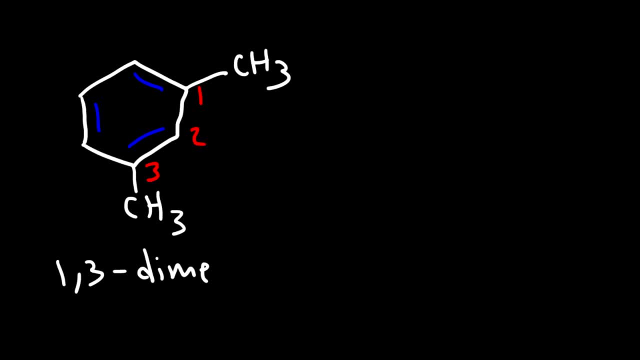 it 1,3-dimethylbenzene, Or we know that 1,3 is the same as meta, so we could say this is meta-xylene, You could write it as M-xylene, or you can actually write out meta-xylene. 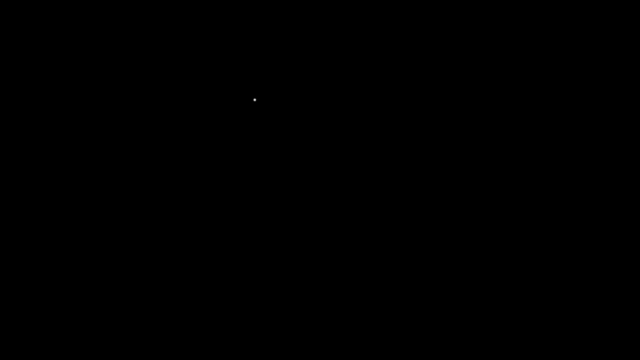 So both ways are acceptable. So what do you think the name for this compound is going to be? So let's call this carbon 1,2,3,4.. So we can call it 1,4-dimethylbenzene, or we know that 1,4. 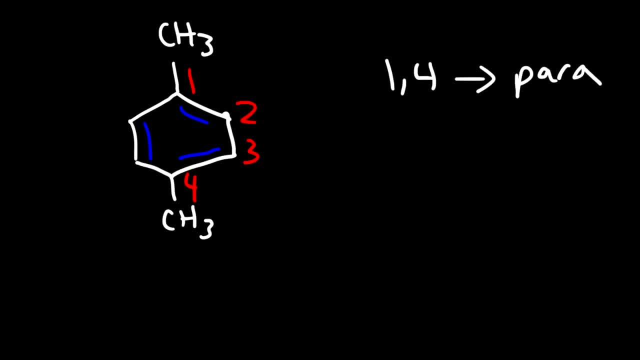 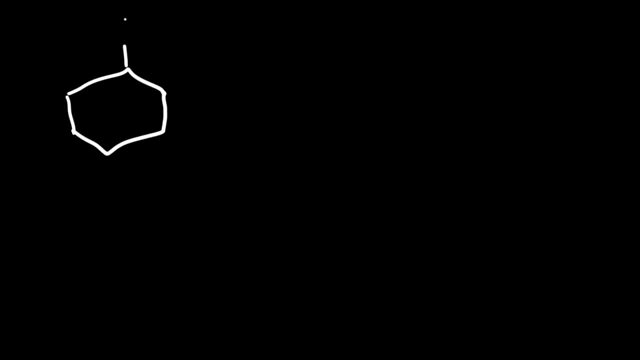 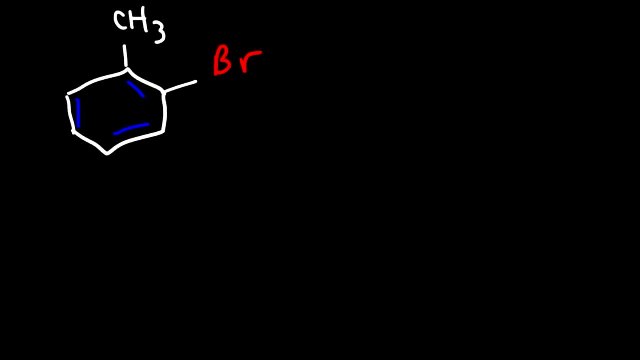 So how can we name this compound? Well, first we need to identify the parent name. We know that a benzene ring plus another group is called toluene, And so that's going to be the parent name. Therefore, we're going to count. 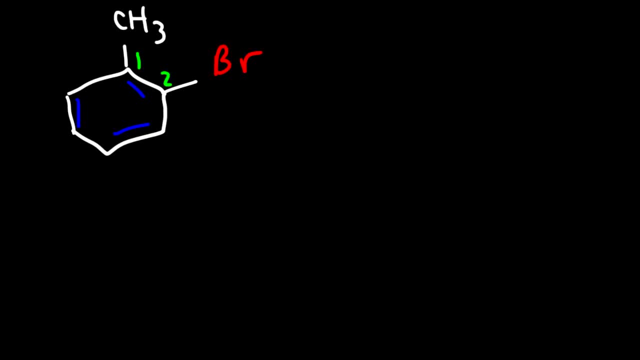 The methyl group is going to be carbon 1, because it's part of the parent name. So therefore we're going to call this 2-bromotoluene, Or we could say ortho-bromotoluene. 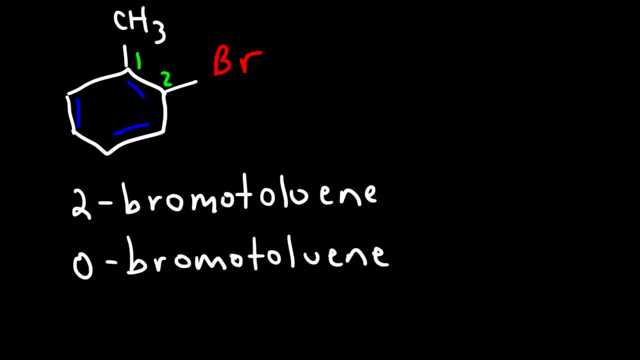 You can use ortho, meta and para for any time you have a disubstituted benzene derivative, That's when you have only two groups attached, groups attached to it. So let's try another example. 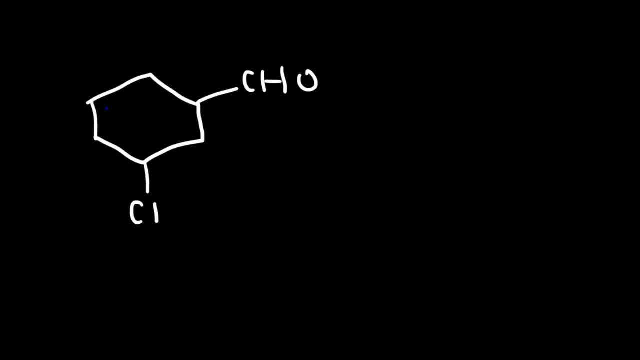 So let's say we have a CHO group and a Cl, Go ahead and name this benzene derivative So a benzene ring with a CHO group that's called benzaldehyde, So that's the parent name, which means that the aldehyde functional group is on carbon. 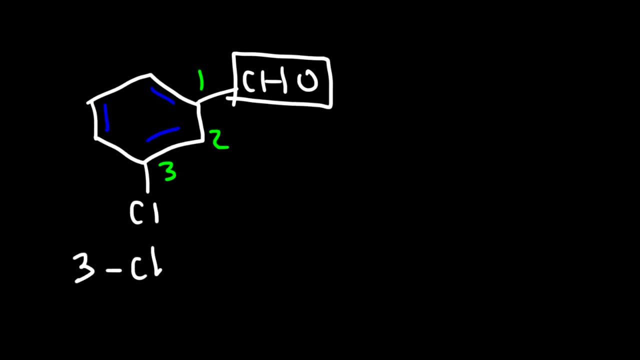 1. So we can call this 3-chloro-bromotoluene, 3-chloro-bromotoluene benzaldehyde, or we could say it's. 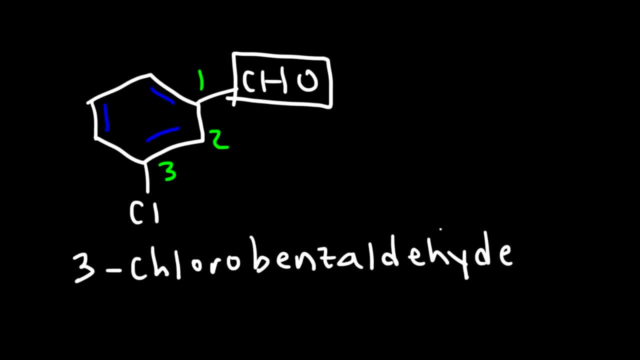 meta-chlorobenzaldehyde, because meta corresponds to the 1,3 positions. Now let's try another example. So let's say we have an OCH3 group and at the same time we have an NO2 group. So what is? 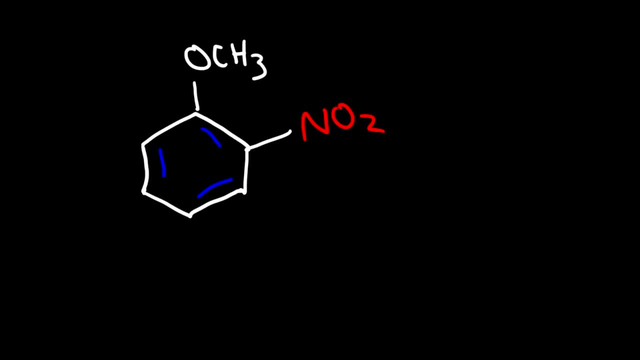 the name of this aromatic compound. So the NO2 group is called nitro and the benzene ring within OCH3 group is called anisole. So the parent name is going to be anisole And the nitro group is on carbon 2.. So we can call this 2-nitro-. 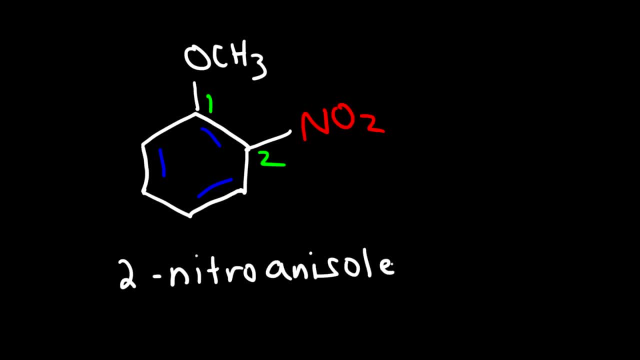 anisole or ortho-nitro-anisole. So now let's move on to tri-substituted benzene derivatives. So go ahead and name the molecule. So the parent name is going to be phenol, because that's the benzene ring with the. 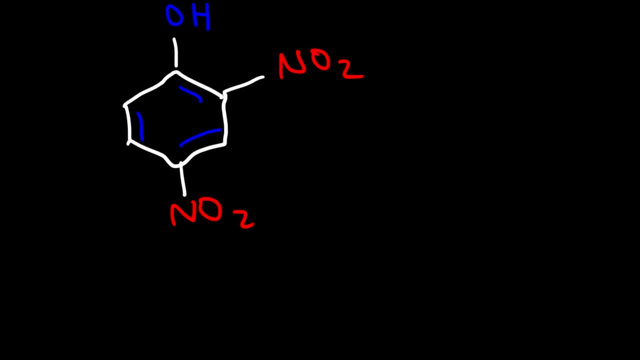 OH group. It doesn't make sense to use nitrobenzene as the parent name, especially when there's two of them, So we need to count this like this, in a clockwise direction, so that we can get the lowest numbers. So this is going to be. 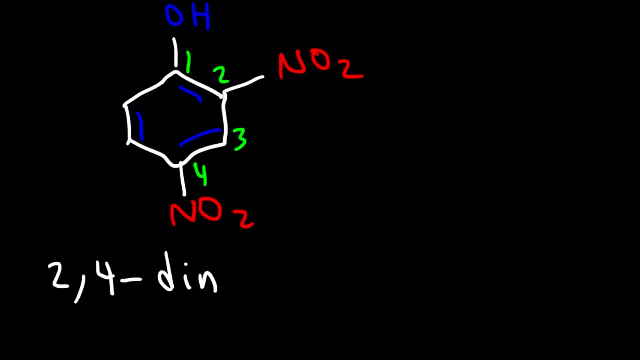 called 2,4-di-nitrile, because we have two of them on carbons- two and four- and then phenol. Now for our next example. we're going to have a carbid-select acid acid, a bromine atom and a nitro group attached to the benzene ring. 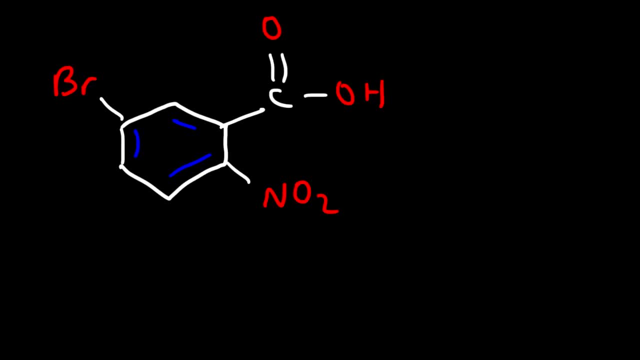 So feel free to pause the video and try this example. So let's start with the parent name. The parent name is going to include the benzene ring and the carboxylic acid, So combined we know that to be benzoic acid, which means this is carbon 1.. 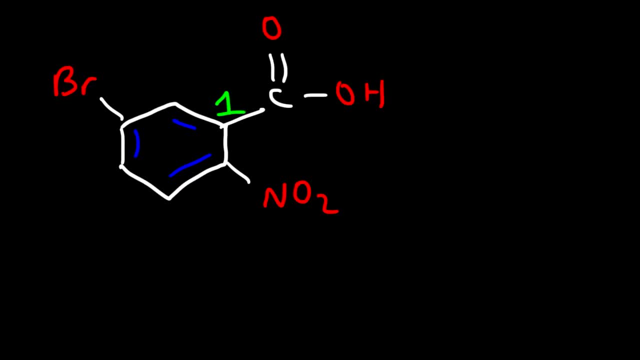 Now, how should we count it? In the clockwise direction or in the counterclockwise direction? So if we try the counterclockwise direction, notice that the bromine atom is on carbon 3 and the nitro group is on carbon 6.. 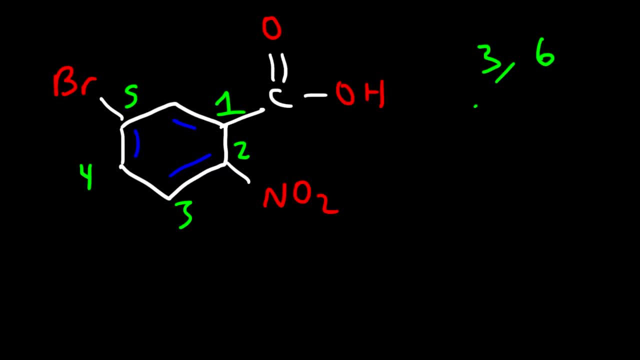 But if we count it clockwise, the nitro is on carbon 2, the bromine is on carbon 5. And so 2 is less than 3, therefore we're going to count it in the clockwise direction. Okay, Now we need to put it in alphabetical order. 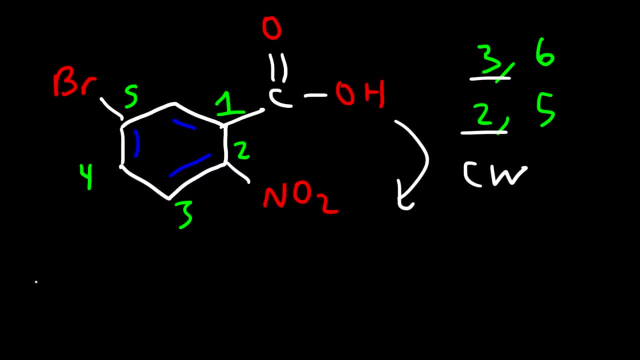 So bromo comes before nitro, So it's going to be 5-bromo-2-nitrobenzoic acid, And so that's how we can name this molecule. Let's try one more example, And so, for this example, we're going to have a bromine atom, a nitro group, and at the 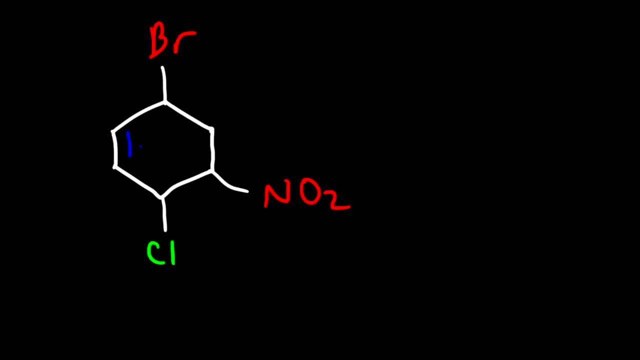 same time a chlorine atom. So what do you think the name of this aromatic compound will be? And how should we count it? Well, if we count it this way: 1,, 2,, 3, 4.. So the numbers will be 1,, 3,, 4.. 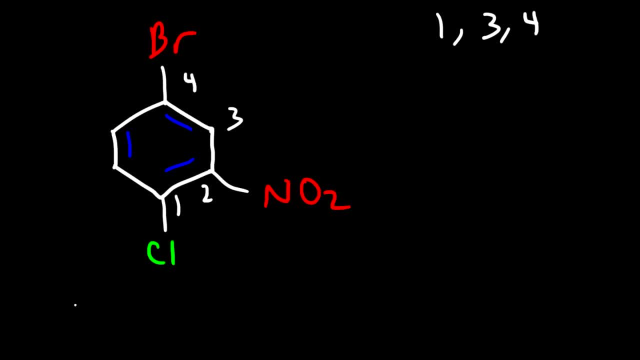 If we count it this way- 1,, 2,, 3, 4.. We will get lower numbers: 1, 2, 4 instead of 1, 3, 4.. And we don't want to start with a nitro group because if we count it this way, this is going. 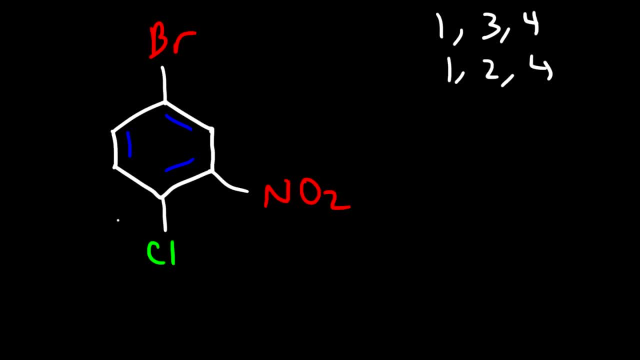 to be 1,, 2,, 5.. And so we don't want that. Or if we count it this way, it's going to be 1,, 3,, 6,, which is even worse. So this is the best option. 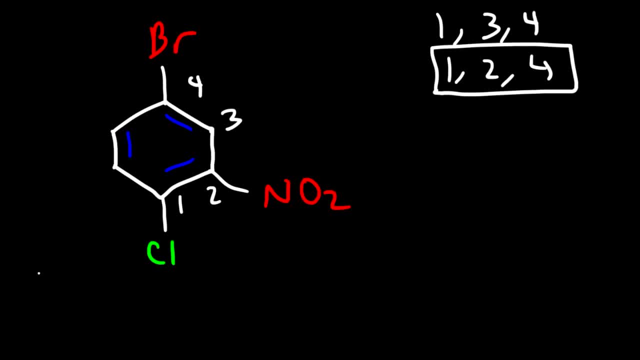 So this is going to be 1,, 2,, 3,, 4.. Okay, Okay, Okay, Okay. Now we have a 4-bromo, We have a 1-chloro and a 2-nitro. 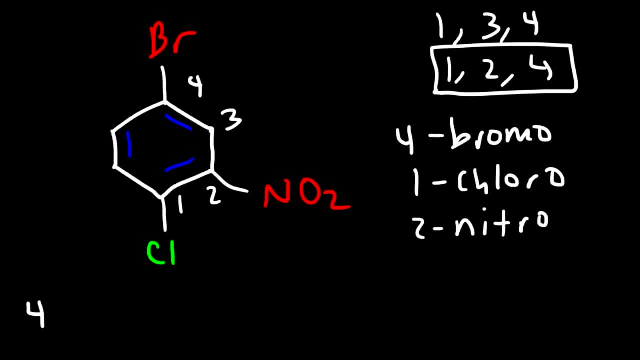 So we need to put the substituents in alphabetical order. So it's going to be 4-bromo, and then 1-chloro becomes C4C, and then dash 2, dash, nitro benzene, And so that's what we're going to do.